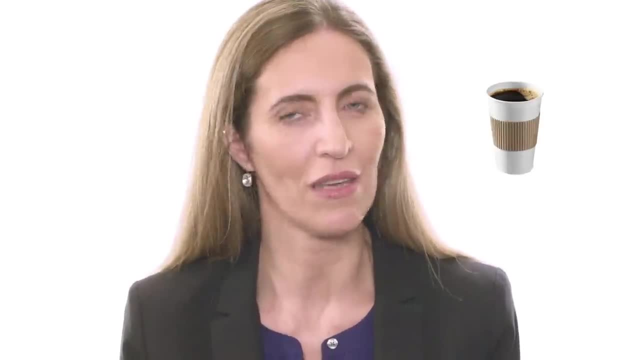 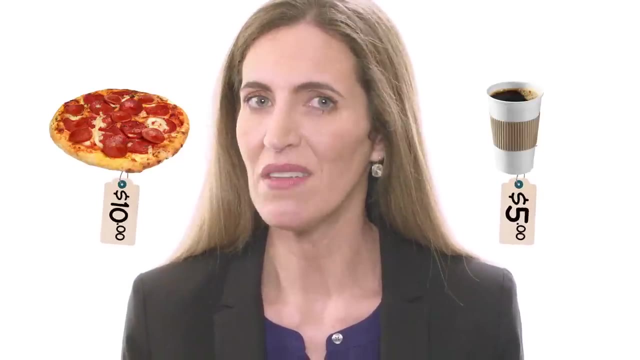 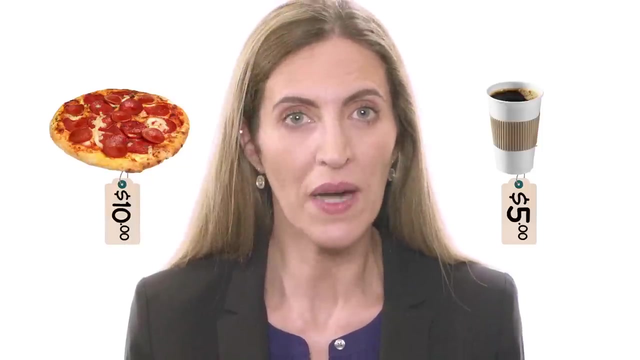 $50 to spend on just two goods: coffee and pizza. Coffee costs $5 and pizza costs $10. So pizza is twice as expensive as coffee. There are several different combinations of coffee and pizza you could buy with this money. Let's plot a few of your options on a graph. 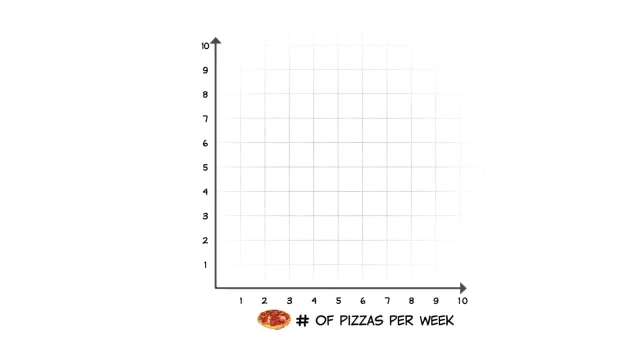 On the X-axis. On the x-axis we have the number of pizzas per week And on the y-axis we have the cups of coffee. per week, You could buy two cups of coffee and four pizzas. four cups of coffee and three pizzas. 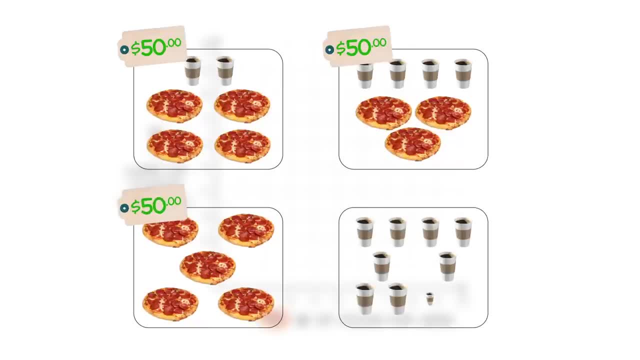 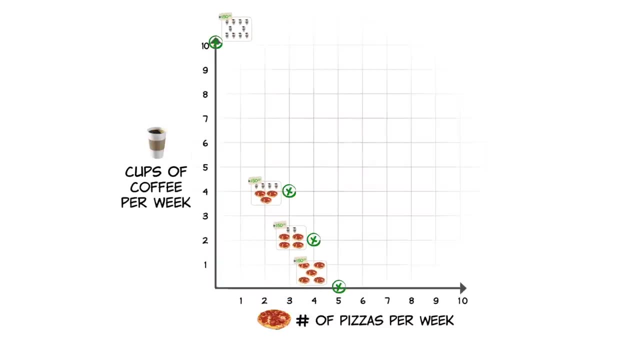 five pizzas but no coffee, or 10 cups of coffee but no pizza. When you connect the different options that represent the ways you can spend your $50, you get a straight line. This is your budget constraint and it represents all possible combinations. 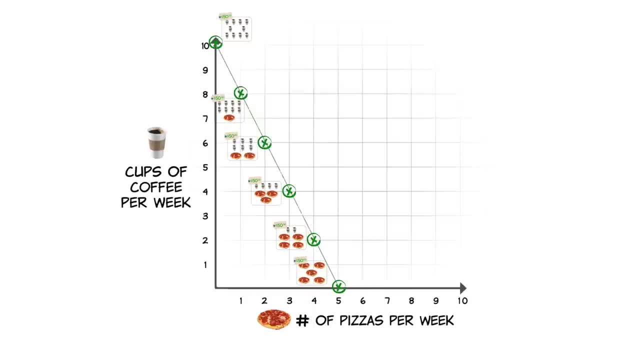 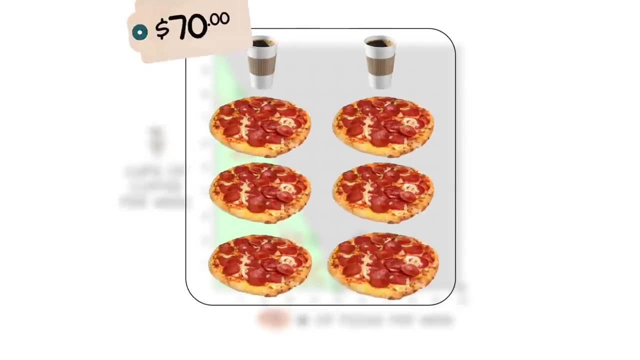 of coffee and pizza you can buy. given your budget and the prices of coffee and pizza, This budget line also separates what you can afford from what you cannot afford. Maybe you wish you could buy two cups of coffee and six pizzas, or four cups of coffee and 10 pizzas. 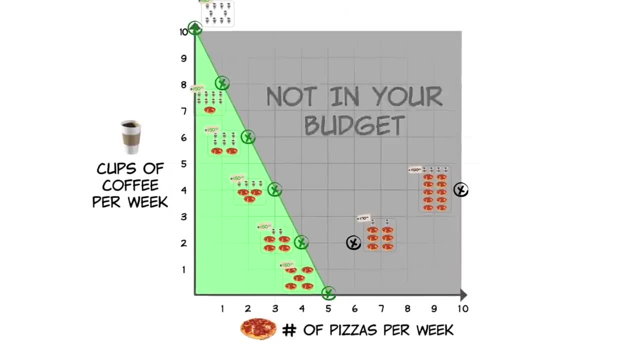 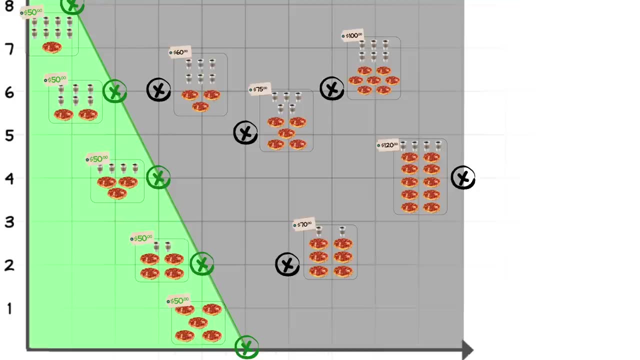 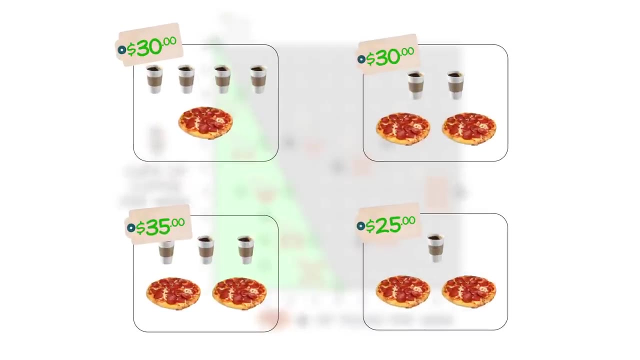 but these are not in your budget, Sorry. All these different combinations cost more than you have, so they're unaffordable given your budget and the prices of these two goods. Combinations of coffee and pizza below the budget line, on the other hand, are within your means. 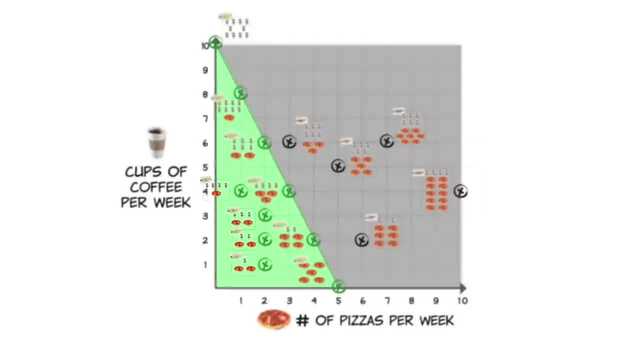 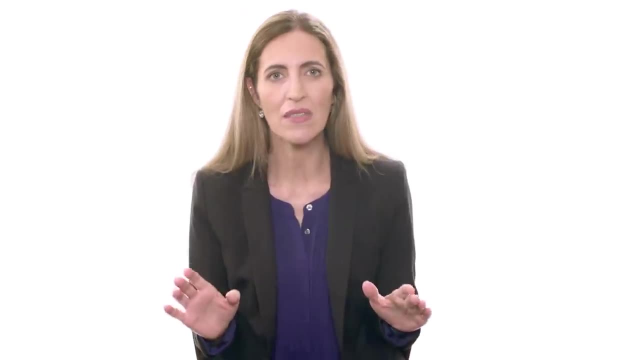 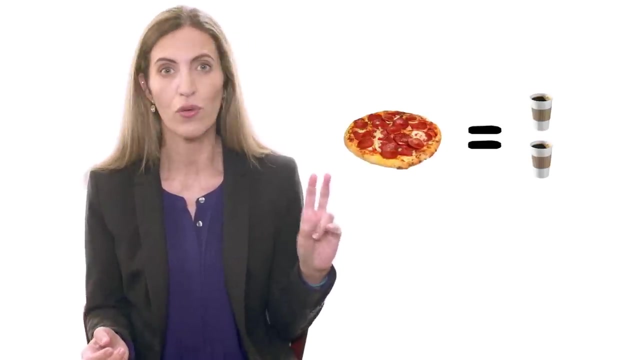 so they're affordable and you could buy them if you wanted. The budget constraint also reflects how the market substitutes between the two goods. Remember, pizzas are twice as expensive as coffee, and this simply means that the relative price of one pizza is two cups of coffee. 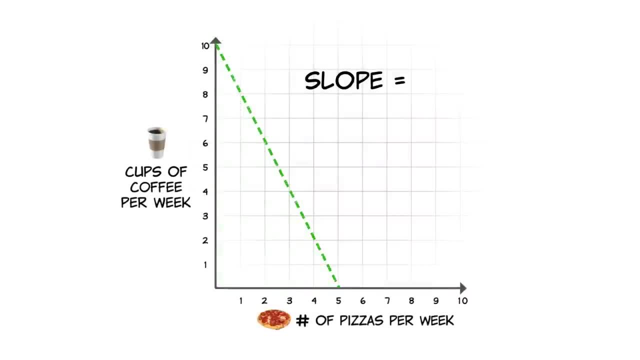 You see this on the slope of the budget constraint, which is two. Well, actually it's negative two, but we're less concerned about the sign, although it does remind us that having more of one good requires giving up some of the other. 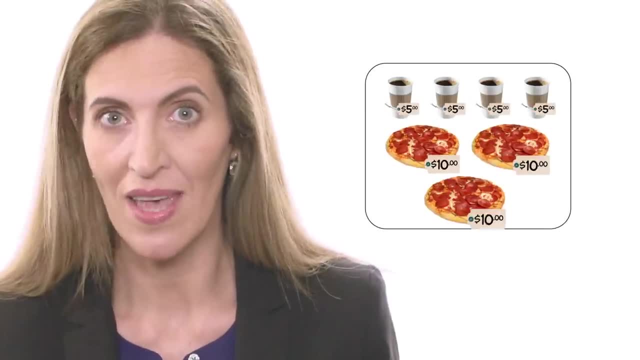 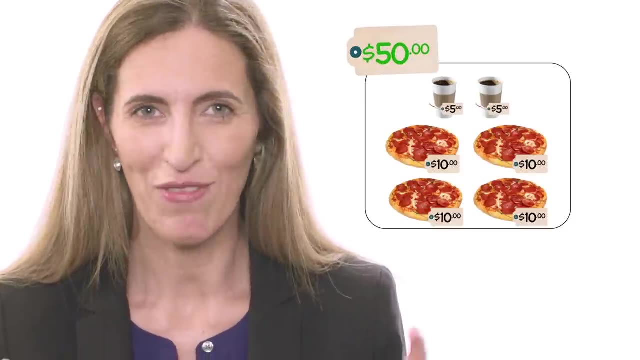 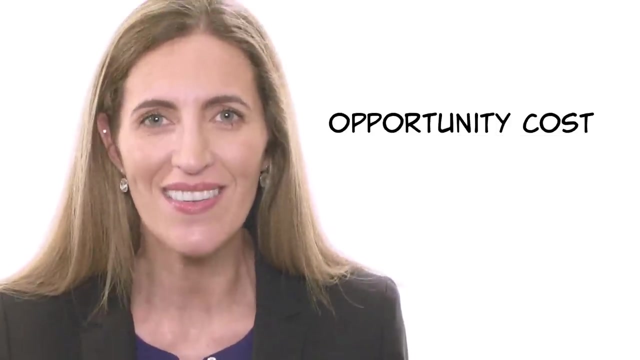 When coffee costs $5 and pizzas cost $10,. if you want an additional pizza, you have to give up. Give up two cups of coffee. If this made you think about opportunity cost, you're right. The slope of the budget constraint is the opportunity cost of pizza. 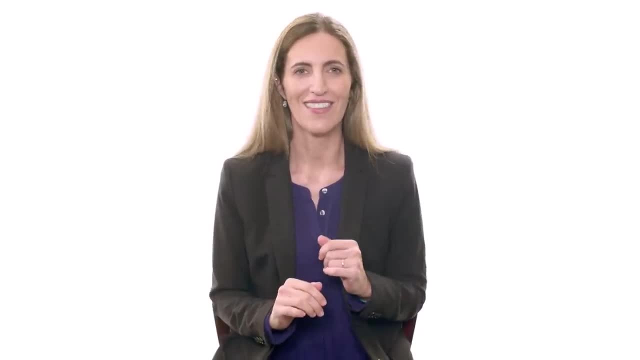 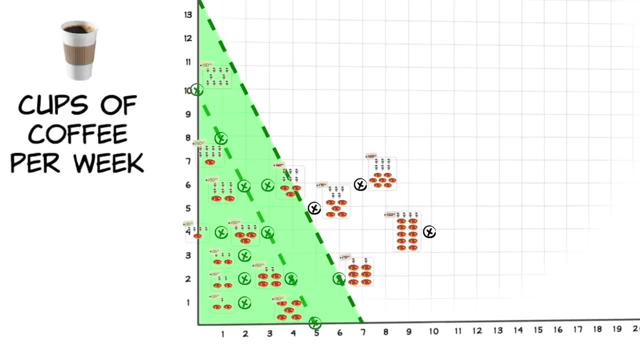 Will this trade-off change if your budget increases, Say if you find a $20 bill in the pocket of your winter jacket and now have $70 to spend on these two goods? No, The trade-off is given by the market's prices. 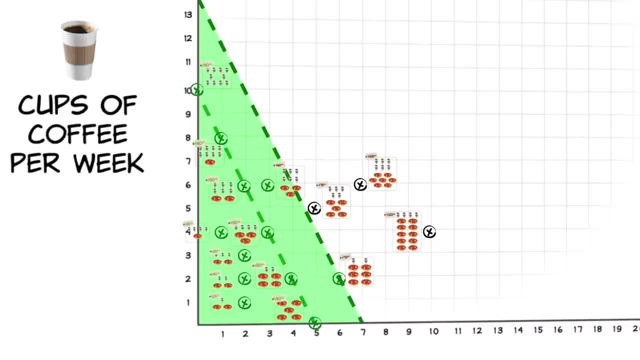 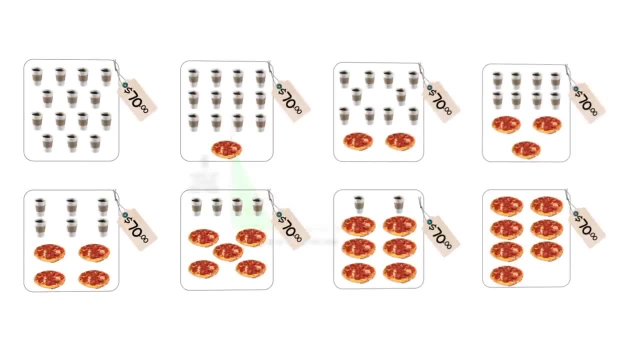 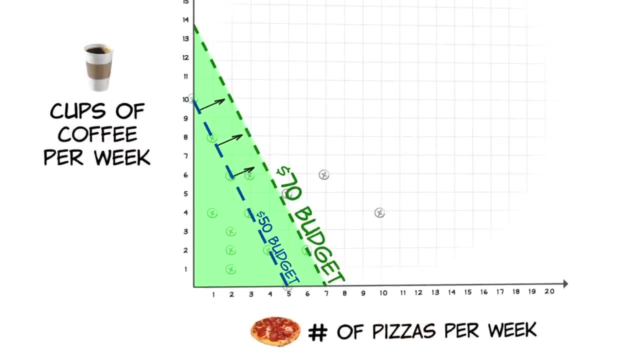 so changes in your income do not affect the relative price of goods. Sure, you'll be able to afford and choose between all of the consumption combinations that total $70, and you can see how this makes your budget constraint shift outward. But the two cups of coffee for one pizza trade-off. 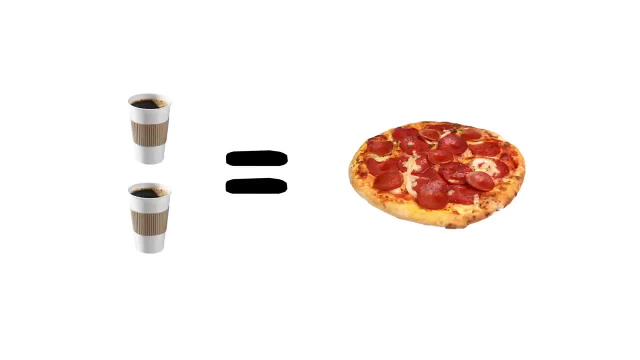 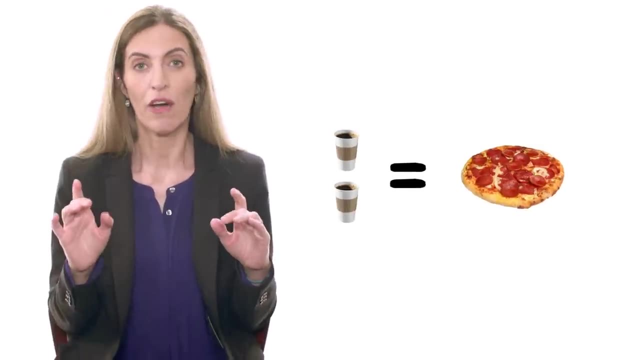 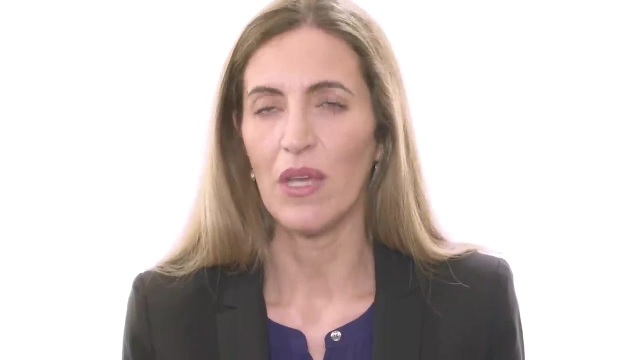 remains the same, and that is because the market still values these two goods relative to one another just like it did before. This trade-off does change if the relative price of the two goods changes. Think of what will happen if, maybe because of unusually good weather- 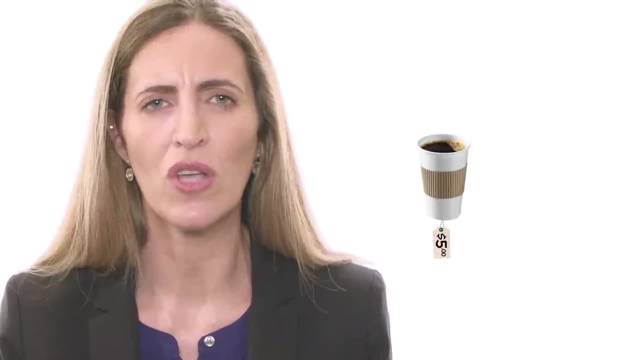 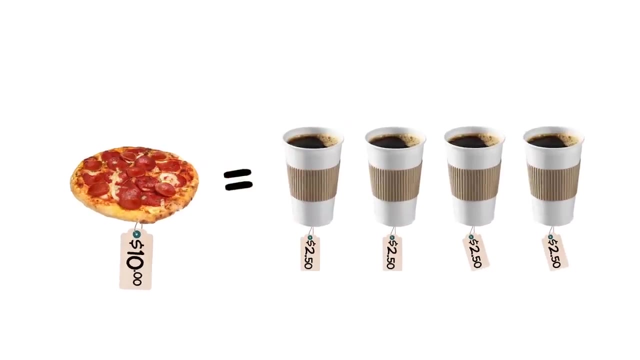 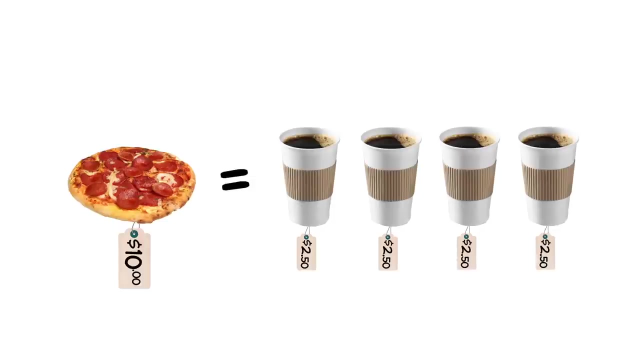 the price of coffee falls from $5 to $2.50.. Does the market trade-off remain the same? No, Pizzas just became four times more expensive than coffee, so you're able to buy four cups of coffee when you give up eating one pizza. 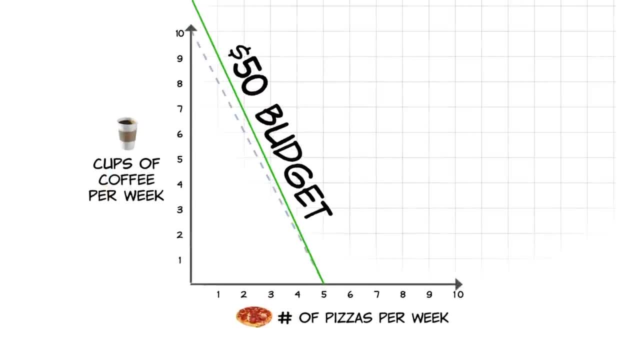 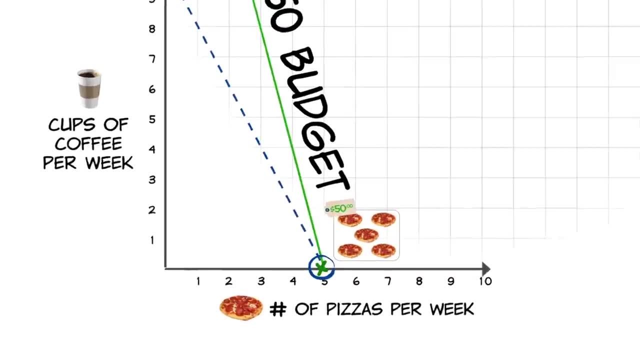 That's right. This will make your budget constraint rotate outward. Notice how, because nothing happened to the price of pizza, the number of pizzas you can buy when you don't buy coffee hasn't changed. You can still only buy five pizzas. But if you spend all of your budget on coffee, 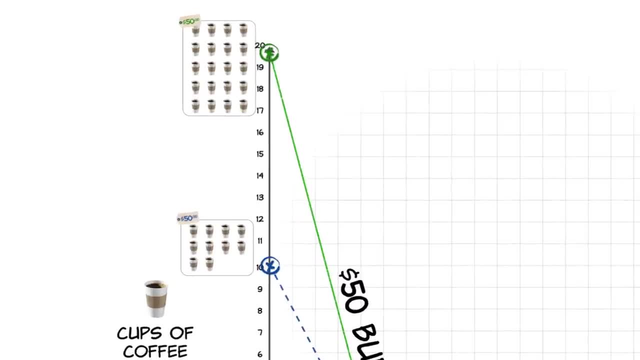 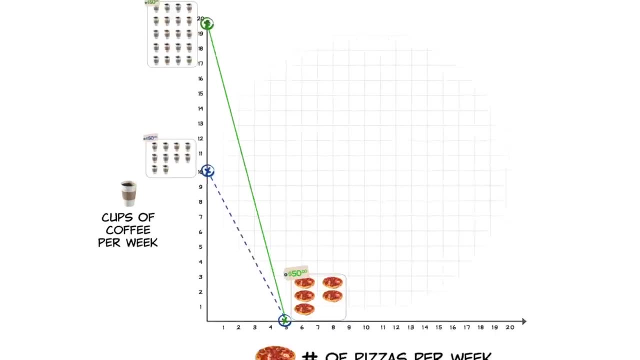 just look at how many more cups of coffee you can buy. You can now buy 20 cups of coffee per week. That's a lot of coffee. That's a lot of coffee. That's a lot of coffee. You see the new higher relative price of pizza in terms of coffee.